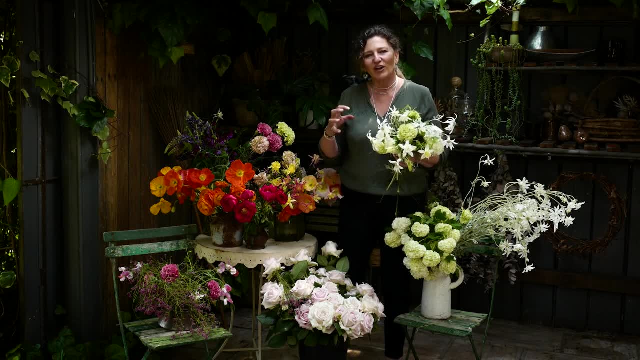 overall cohesiveness of your design, And it's not just colour within the design itself and the way the flowers talk to each other, but it's also acknowledging and understanding how that colour palette works within the space that you're in as well, and the room and the 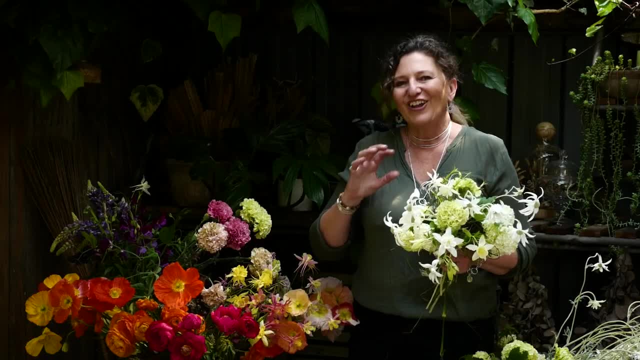 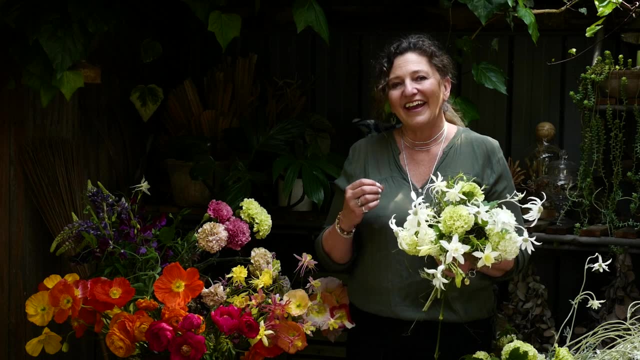 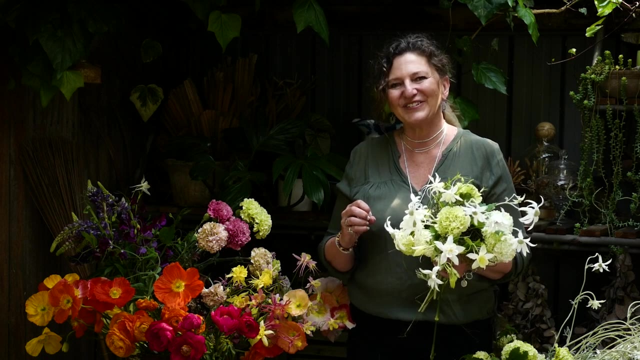 overall aesthetic where this design is going. Lots to talk about here. I used to teach this at a Certificate IV level in college and we would talk about colour for a whole term. So I'm attempting today to condense this into some short, sharp- you know little- demonstrations. 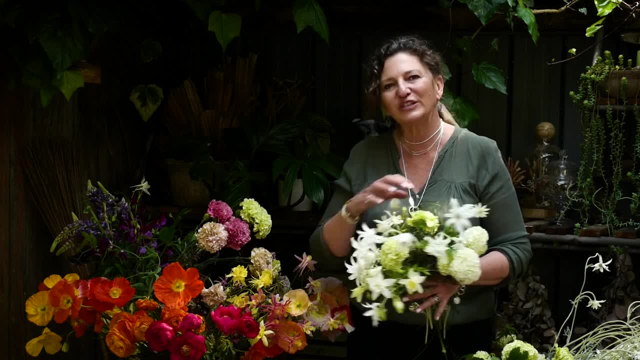 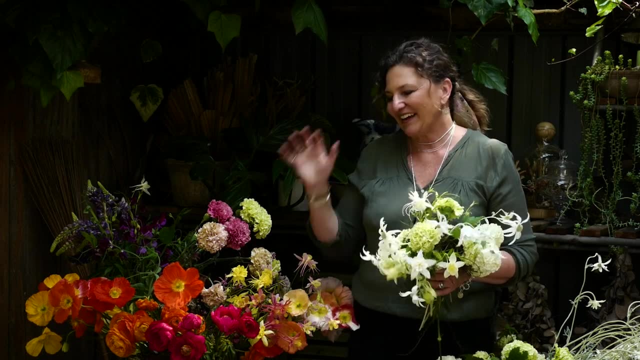 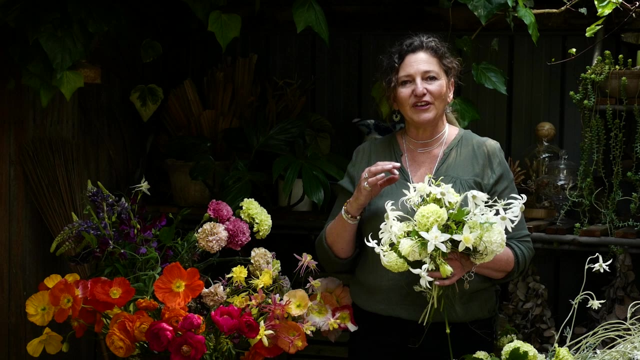 and conversations around a very simple bouquet, because I want you to see those colours actually in an arrangement, albeit a very simple design. So let's get started. First of all, I wanted to talk to you about monochromatic colour harmony. Now, if you haven't got a colour wheel, I highly recommend that you get one As a 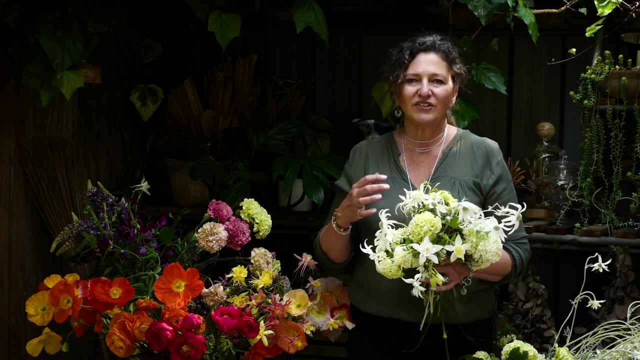 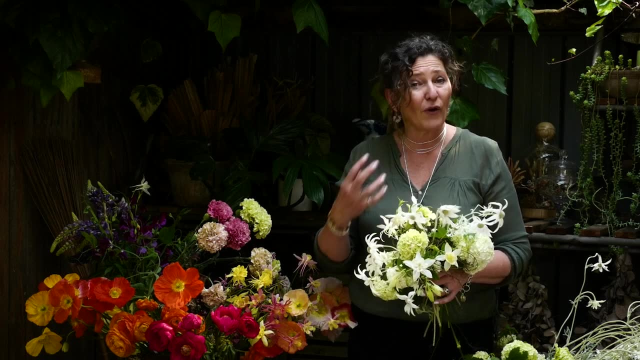 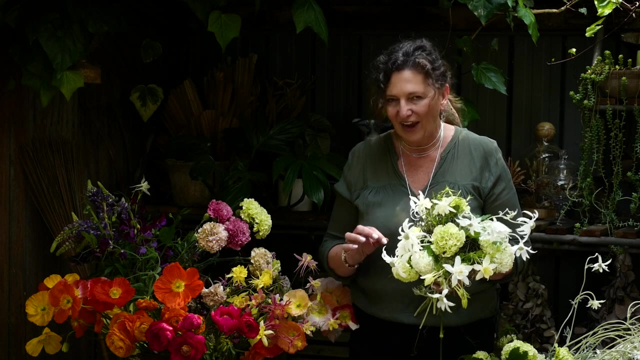 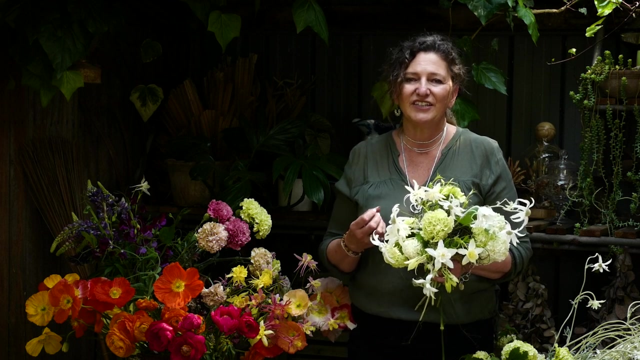 designer, you really need to understand the way colour works, the way it speaks to people, and also how to use it well and how to be brave with your colour. It's important that you understand how colour works, So I have added design notes in this one, a very comprehensive document that you can. 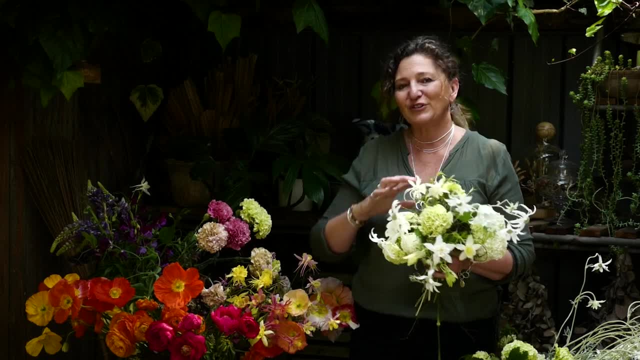 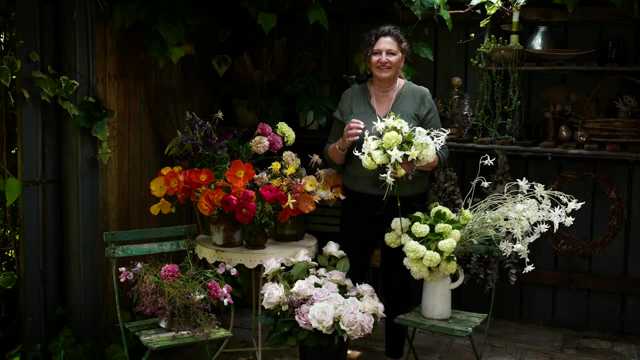 download about colour and colour harmonies. So if you're not sure about anything that we talk about today, make sure that you have a look at that as well. So, first of all, we're talking about a monochromatic colour harmony, and mono meaning one. Now this: 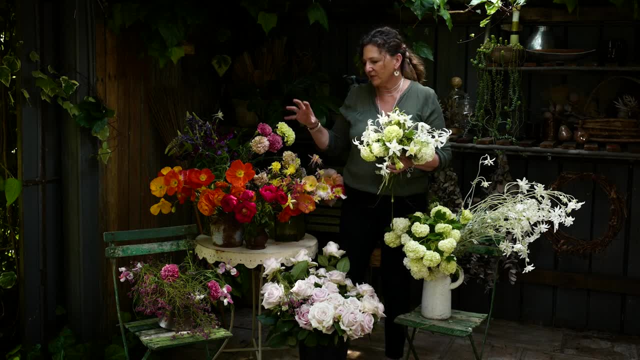 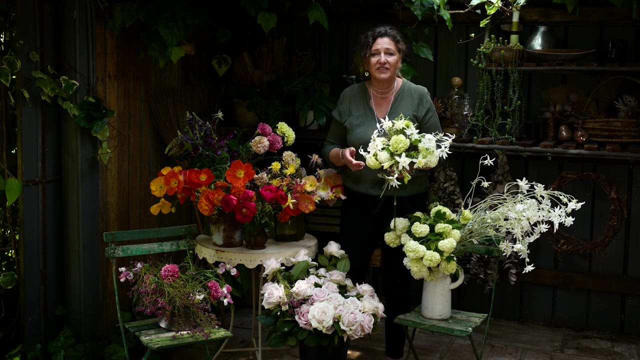 can be in regards to, you know, pinks or blues or yellows or oranges. It doesn't matter what colour it is, As long as you're moving from a pale to a dark tone of the same colour or of the same line on the colour wheel. But we also talk about that in regards to mono being, say, a 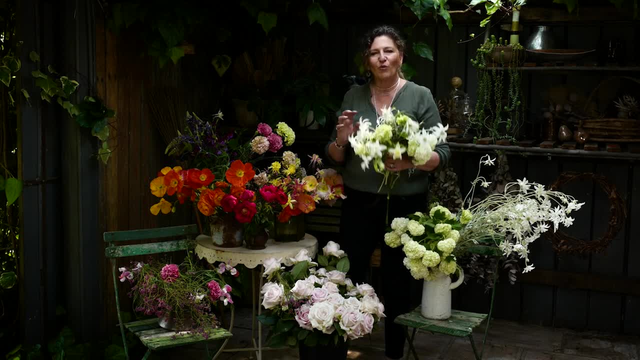 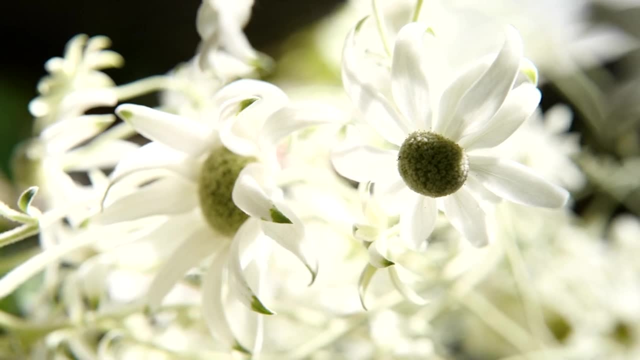 white and green bouquets. Now, not to confuse you, but white actually isn't considered a colour on the colour wheel, It's a neutral. White, grey, black are all neutrals on the colour wheel, which means that you can add white and grey and black to any colour you. 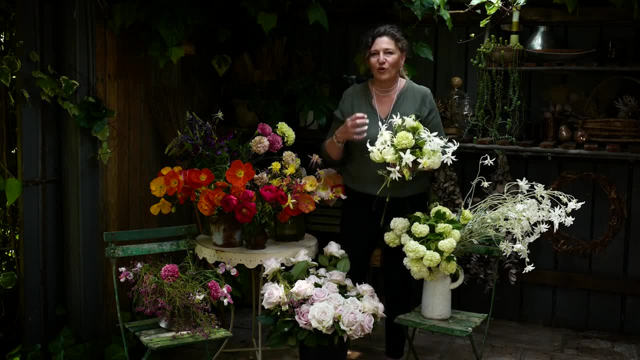 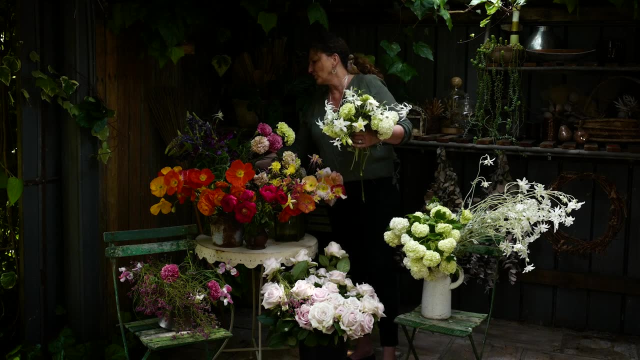 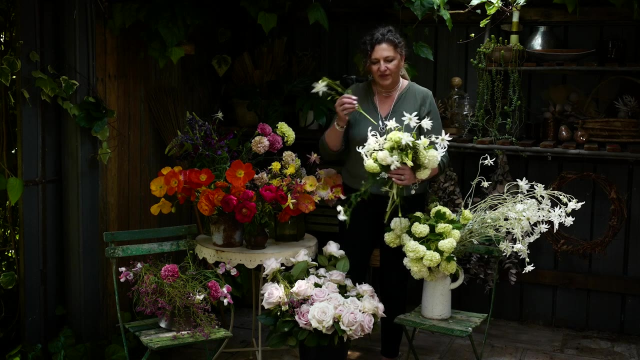 want any colour harmony and it won't be incorrect or it won't be wrong. But to start with this conversation, I wanted to show you a monochromatic bouquet of just whites and greens, And I've, just as I said, just made it really, really simple. We've 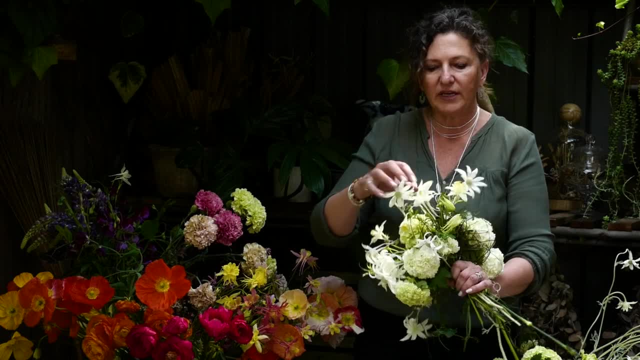 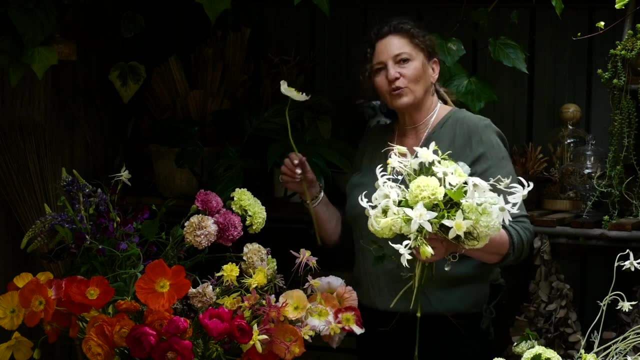 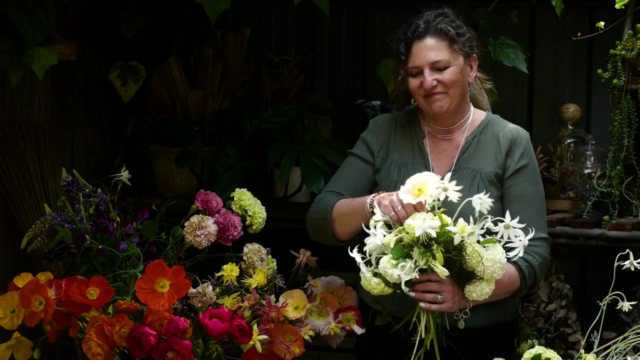 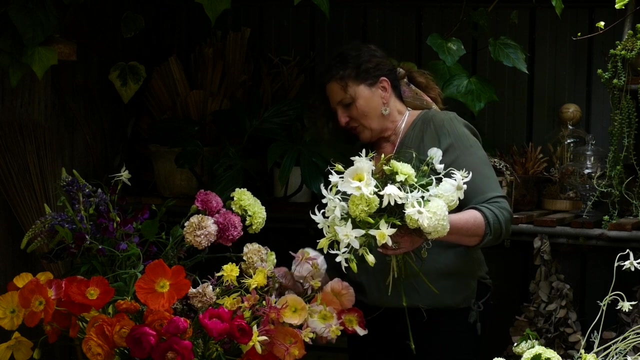 got variations of that green into a really bright white, but also, you'll see, there's a tiny little bit of yellow in these And that talks beautifully to the white poppies. So even though we're we're maybe dancing with breaking a rule, I did want to just show you by bringing in another white. essentially, 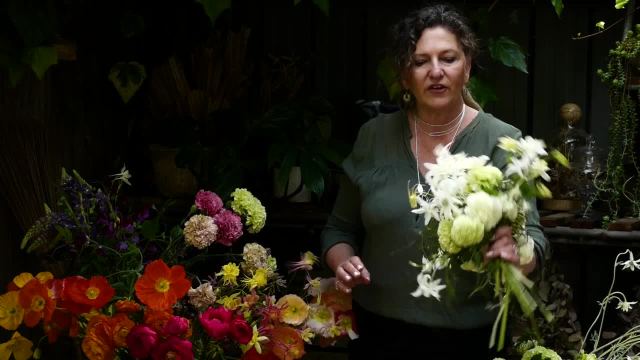 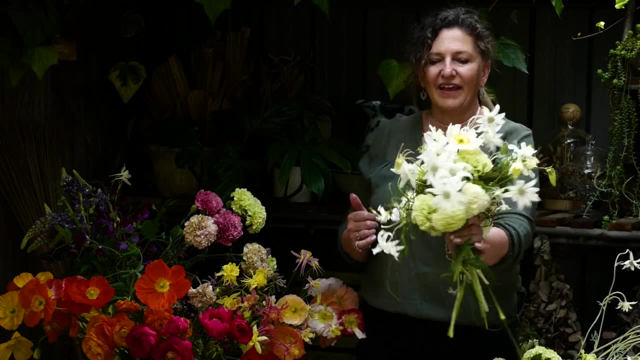 that has that little hint of yellow, then that picks up the little bit of yellow. So this is a monochromatic bouquet of yellow in the aquilesia Still means it's monochromatic and it still means that it is a you know one colour harmony bouquet. 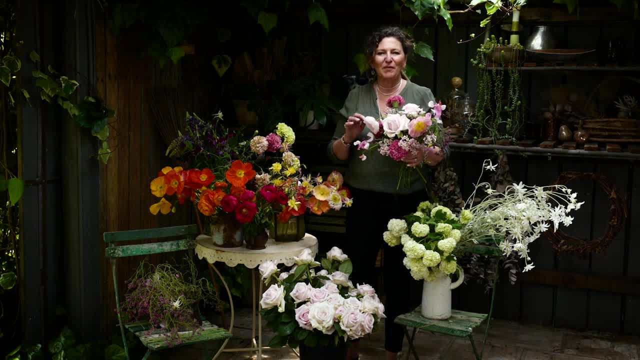 Okay, so I've wanted to also share with you a monochromatic in a colour. Now that I've showed you the monochromatic in a neutral, I wanted to make sure that you understand what monochromatic means. And this, personally, this is the colour harmony that I gravitate. 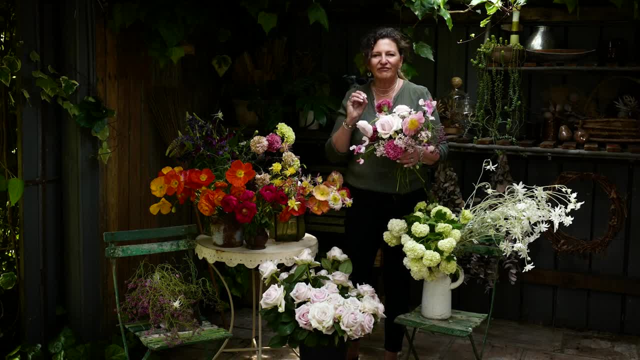 towards the most Once I have one particular flower, it just could be one or two, it could be three, it could be four, it could be five, it could be six, it could be seven, it could be eight, it could be eight, it could be nine, it could be ten, it could be ten, it could be eleven, it could be. 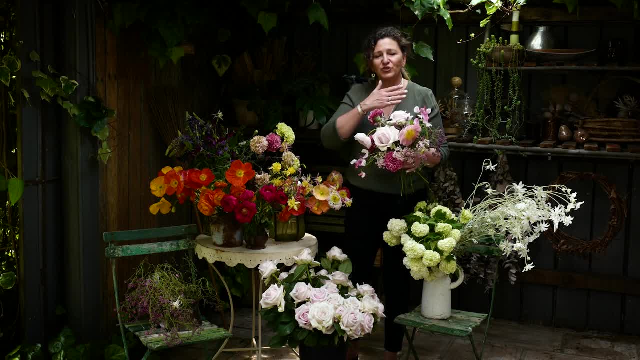 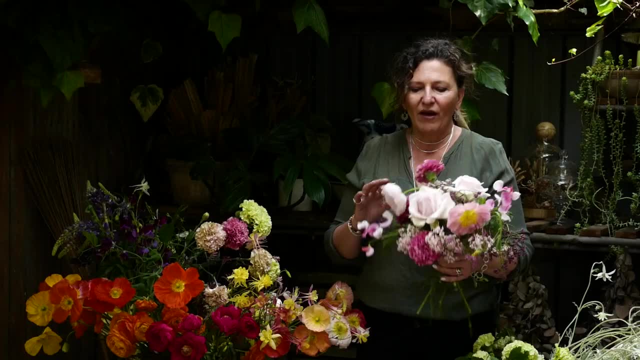 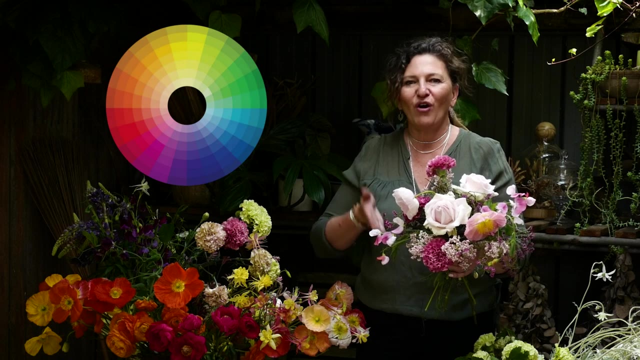 nine. So I'm gonna show you one element and then it's just natural for my eye to move to a darker or a lighter shade and tone of that one colour. Now, this obviously is pink, And you'll find pink on the red quadrant of your colour wheel. 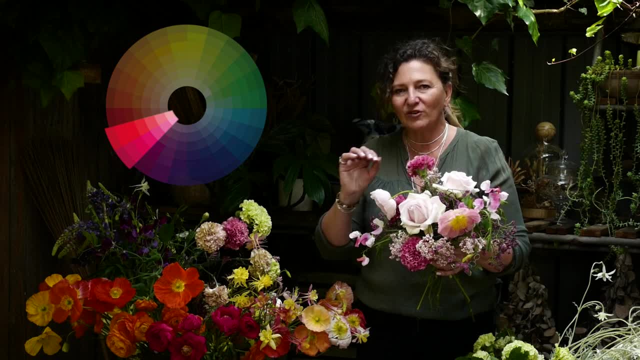 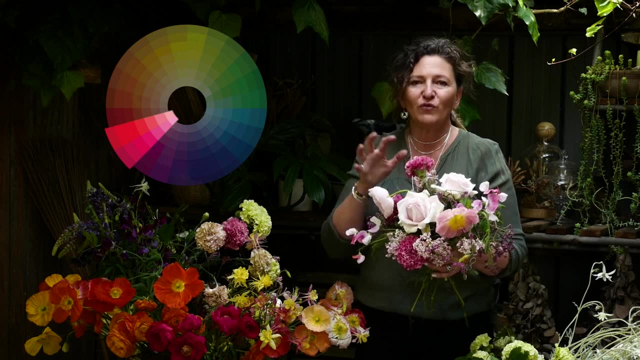 And you'll see that your red once you add white, and you add a little bit more white and a little bit more white, You move into that pink and then, if you add a little bit more black, little bit more black, you move into that burgundy and those darker, dusty pinky tones and that's. 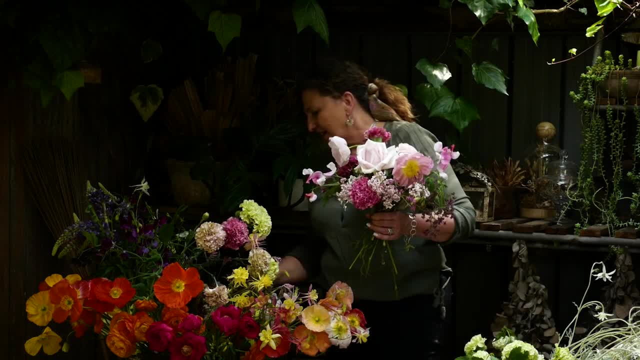 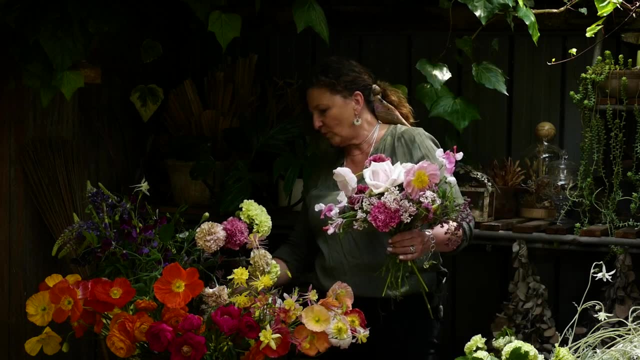 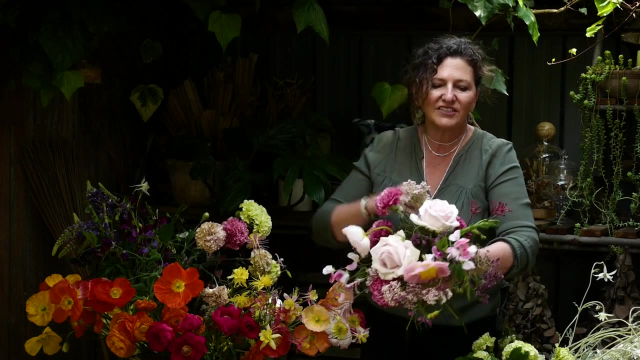 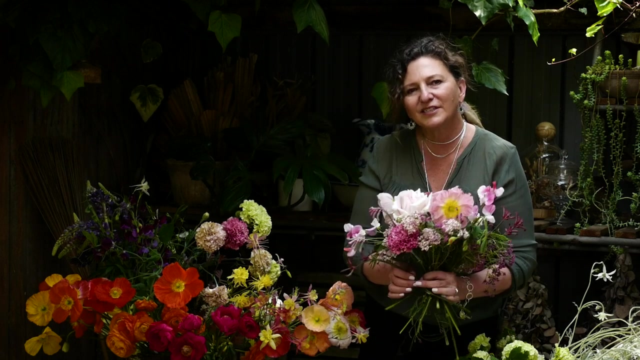 essentially what this is here: a monochromatic color scheme in a pink tones and even bringing in this kangaroo paw, you can see, then I can also bring in this darker burgundy kangaroo paw and then that ties in really beautifully with the darker status. So, as I said, this, this one, probably appeals to me. the 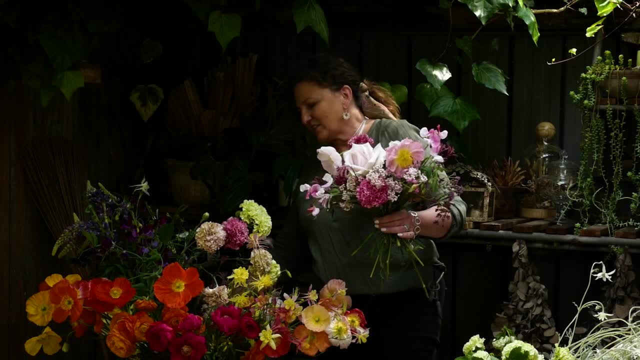 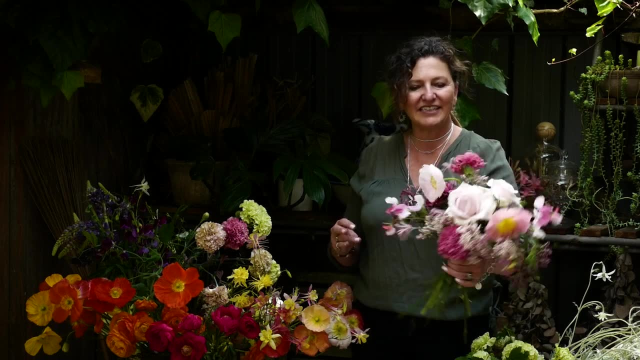 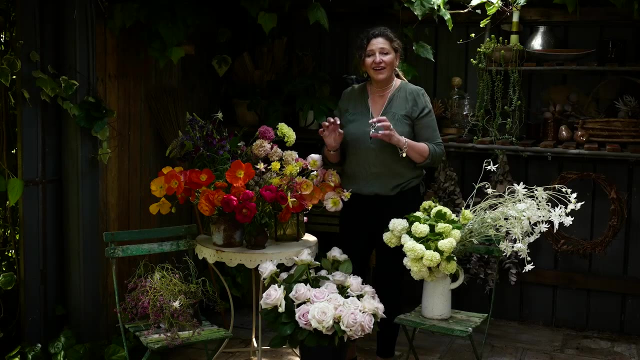 most, I would say, out of every color, harmony. it's just one that I just kind of- I don't know my eyes like it, I guess, not necessarily pink, but just that sense of moving with one color, but darker and lighter tones of that one color. Now I'd 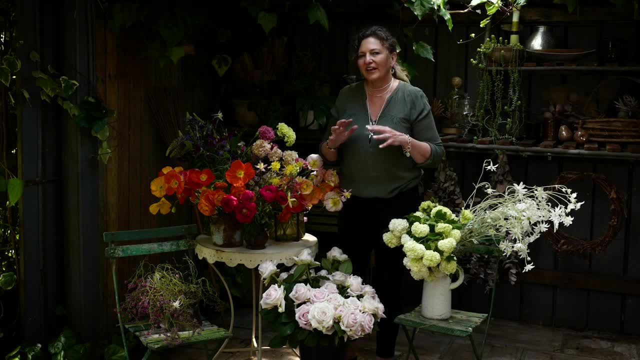 like to share with you my thoughts on, not necessarily a color harmony, but a rule that I think you should really consider when you're putting your bokehs together. Now, within the realms of color, we have bright, what we call hot colors, and we also have pastels of that same. 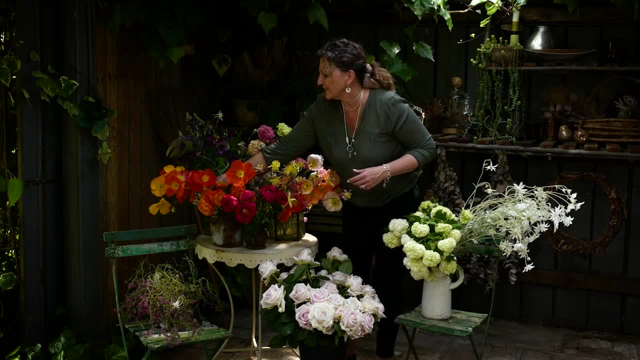 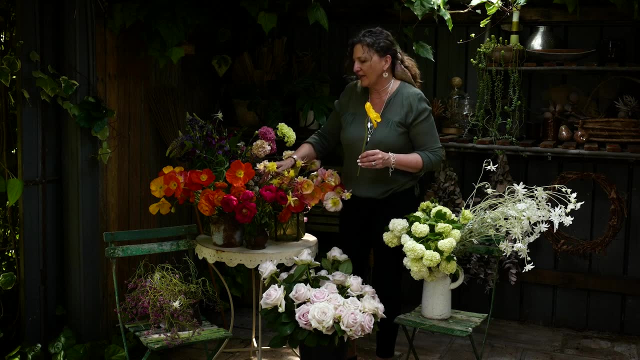 tone. so if you can imagine, you know yellow. yellow is a classic example. I've got a hot, bright yellow poppy here and then I've got almost buttery pastel yellow aqualiges. you can see how soft they are Now. as a rule, I think you. 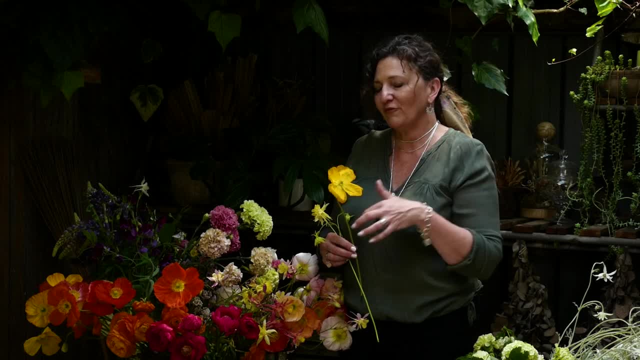 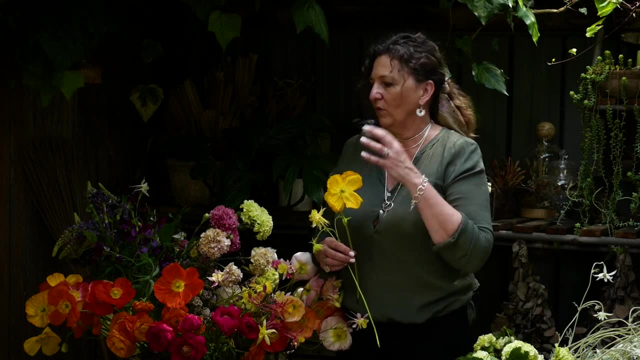 should really consider that once you've got your bokehs together- and you've got your bokehs together and you start- you've made the decision to work with hot, bright colors. stay there. it doesn't mean that you have to have all yellow or all orange. some of the most beautiful color combinations are right here, where. 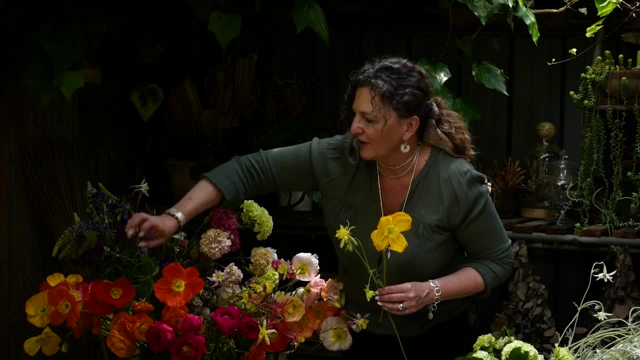 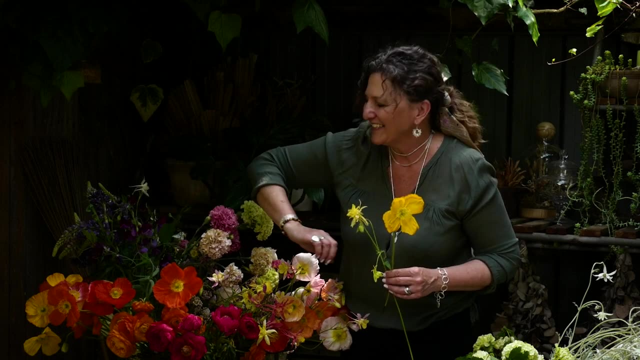 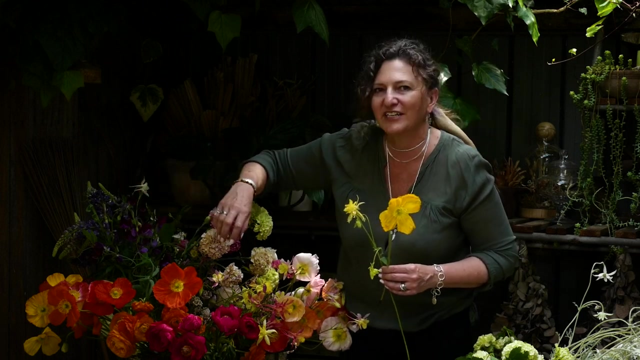 you've got hot purple, hot orange, hot yellow, hot pink. you can see how dynamic that is, and every flower is having its moment in the Sun, so to speak, and every flower is shining. no one is taking over anyone else, they're all. they're all fighting for your attention, but they're doing it beautifully together and the 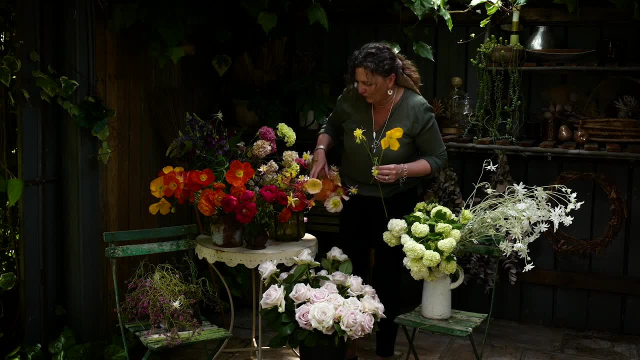 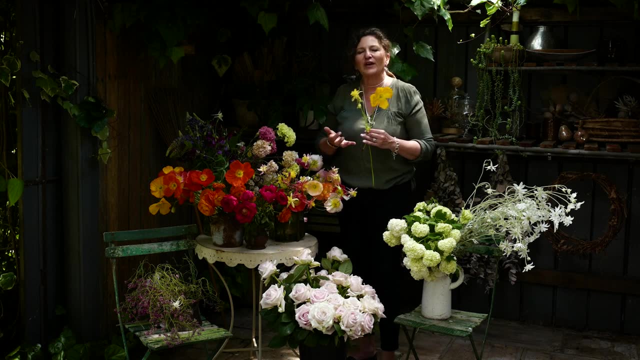 same with your pastels. you know, when you've got these beautiful pastel tones together, you can see how lovely and cohesive they are together. you know, think about mauve and pale pink and butter yellow and apricot. all of those tones are beautiful together too. the mistake I see people making is once they 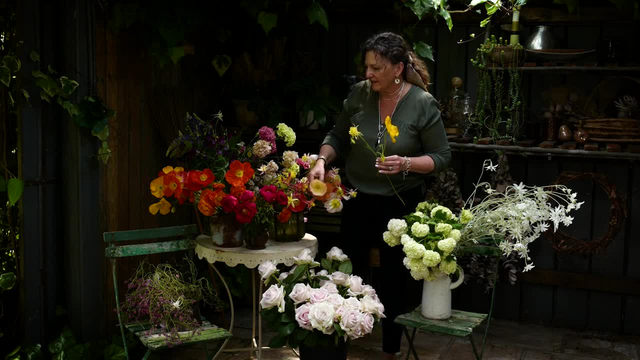 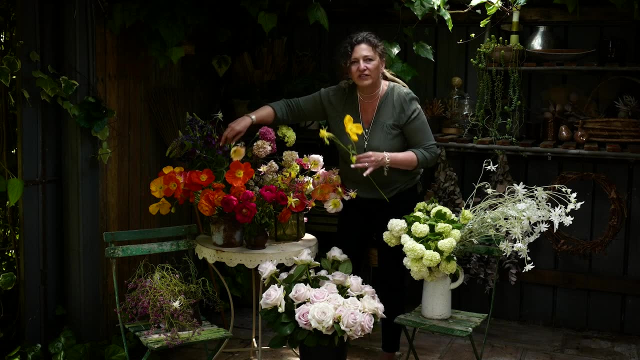 go into this hot realm and then you try to add in. you know these pastel tones. you can see that they just gray out, they just disappear, they don't sing at all, they just completely wash out, whereas if you've got all your pastels together, they 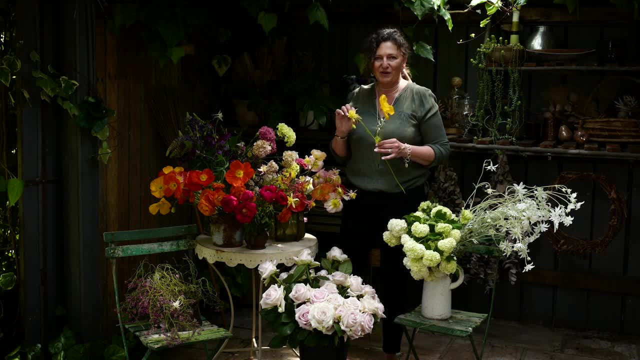 all sing. you've got all your hot colors together and they do as well. there's only one, I guess, area that we can break that rule, and that's if we go down the monochromatic road, and that's when, say, we were instance using yellows, we can go. 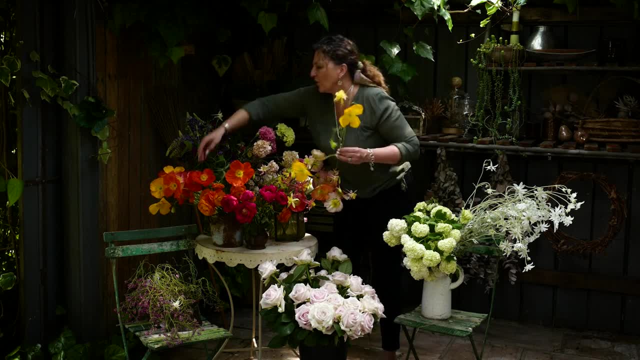 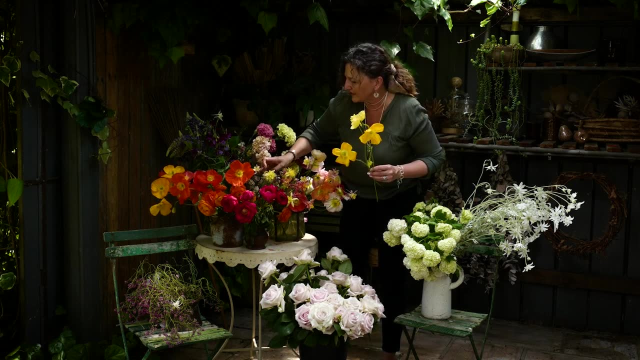 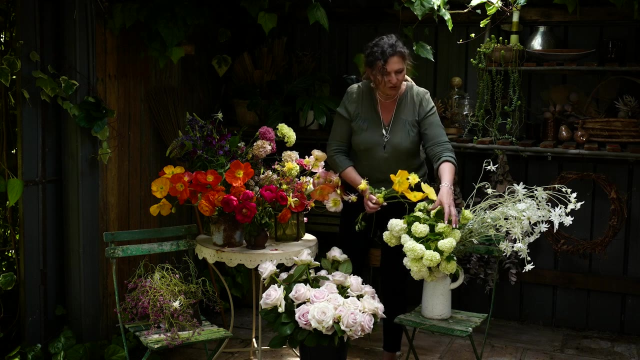 yellow. we've got that bright yellow. we're going to move into that paler yellow and into- you know this- aquilegia, then into say, you know almost greeny whites, and you can see that that can work beautifully together. so pastels and brights only when you're in a 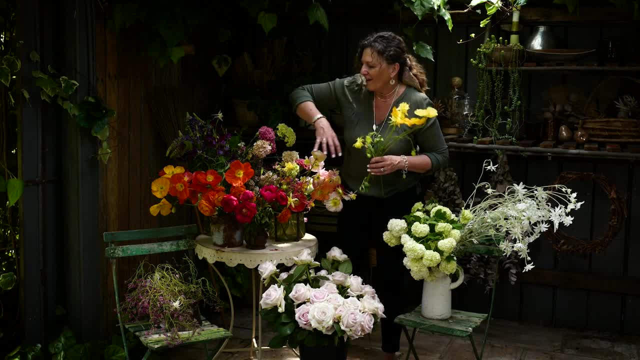 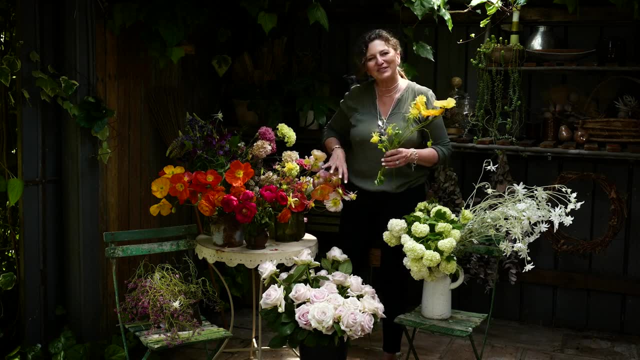 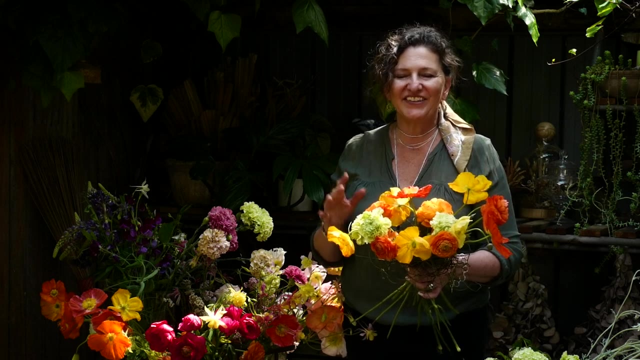 monochromatic color harmony. every single color if you want to stay in your hot realm, and every color if you want to stay in your pastel realm. I hope that makes sense. now we're looking at the analogous color harmony, so this one on the color wheel is the three colors that are directly adjacent to each other. on 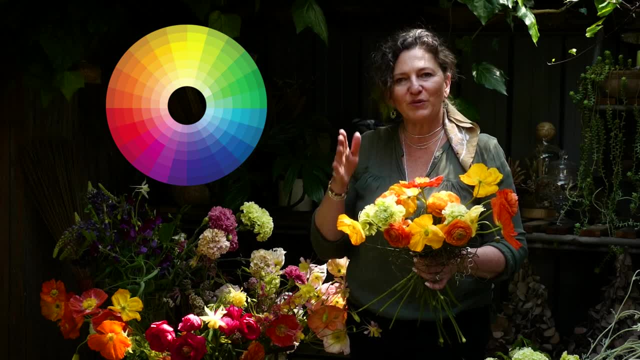 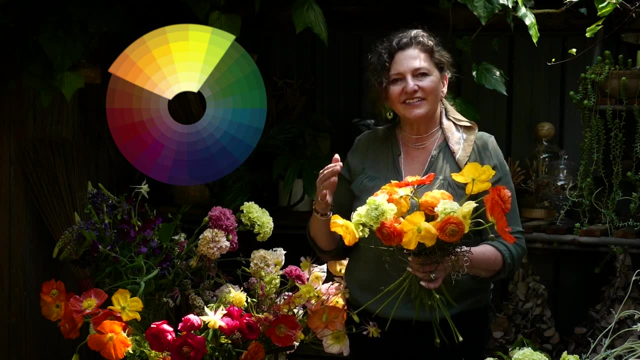 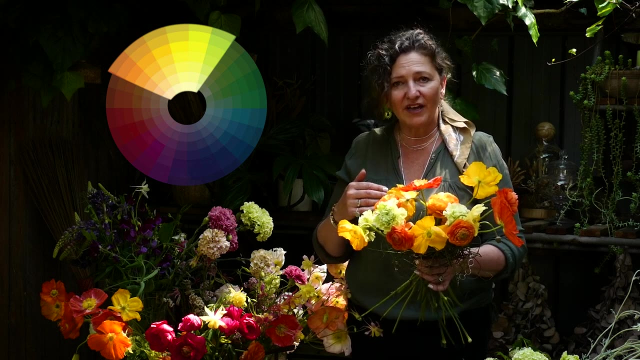 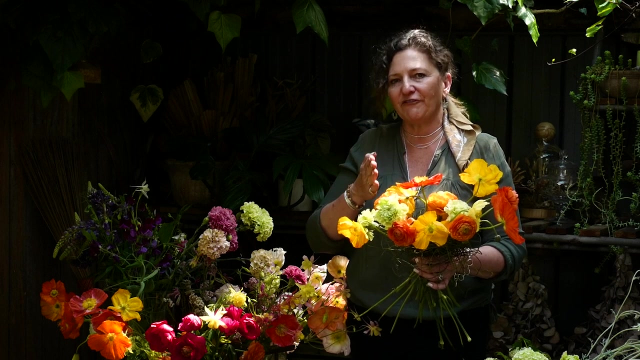 the wheel. so it can it. for this instance, we're looking at orange to yellows, to lime, yellow into green, and they're the three that run beside each other. they can still be lighter and darker tones of those colors. they don't all need to be hot, but they. you see that they're definite different colors down on the 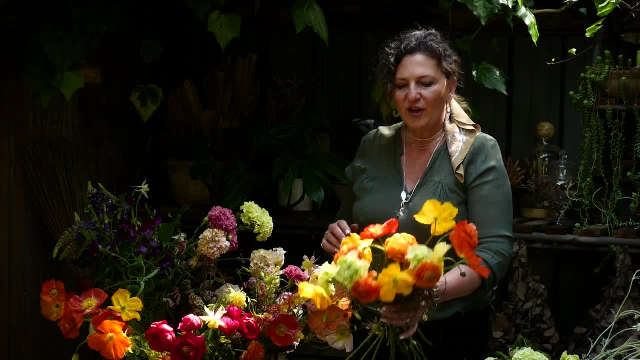 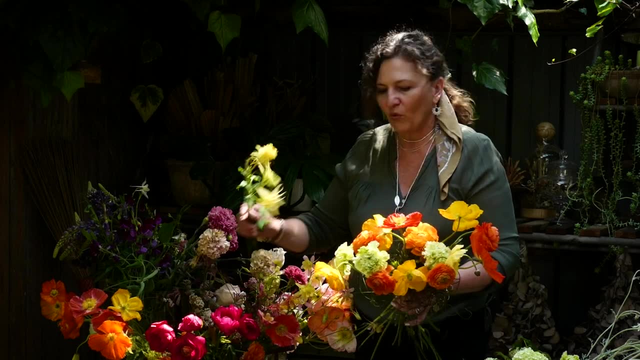 wheel. so we've got orange in the ranunculus and the poppies moving into a darker yellow and then a pale yellow and then bringing in a little bit more of that limey green with the carnations and the columbines. and another thing to. 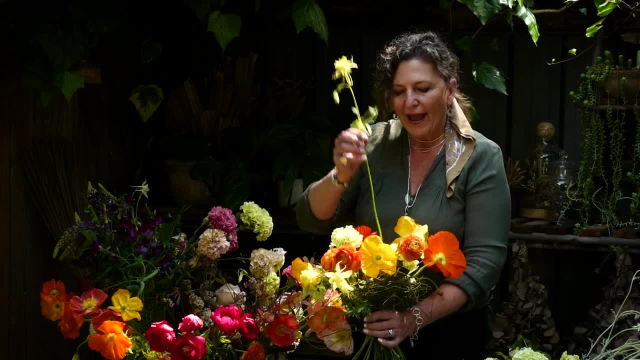 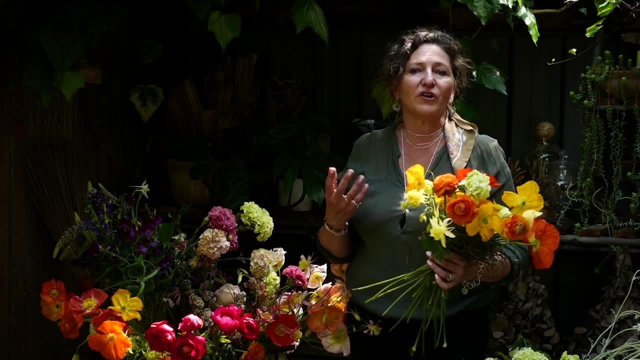 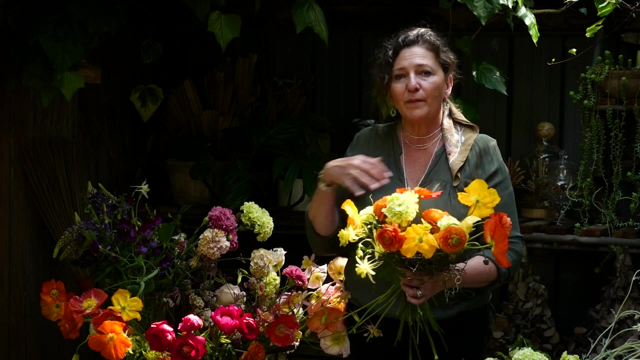 consider too is that you can bring in your wrap and your ribbons to change that color harmony, so you might find that you've got a bouquet that's almost all orange, but then when you wrap it with lemons and green and limey green, you're actually creating a whole bouquet. 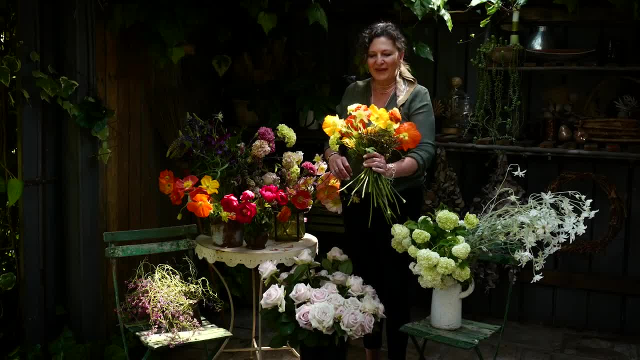 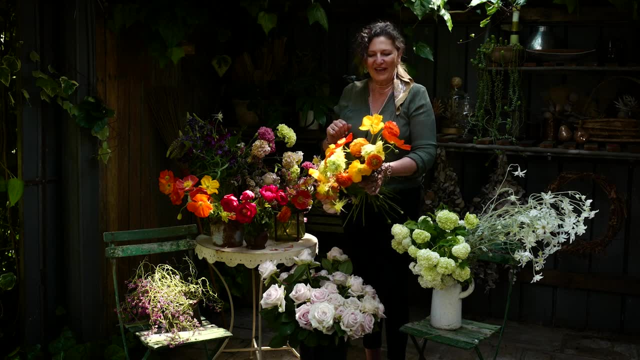 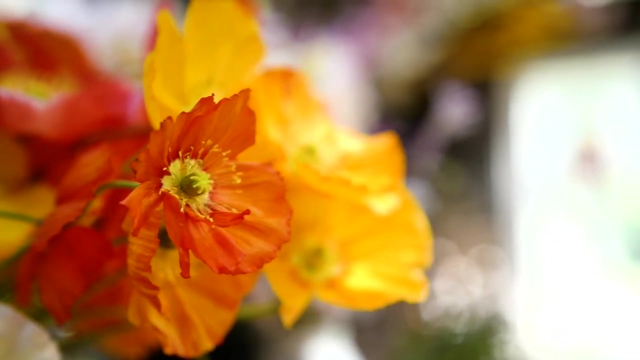 that's an analogous color scheme. so you know, for me orange is actually one of my least favorite colored flowers, if I can say that. but when I have it in a color harmony like this, where it's talking to these other elements and you can see, you know, those tones work together. I think that just makes orange sing. I just like. 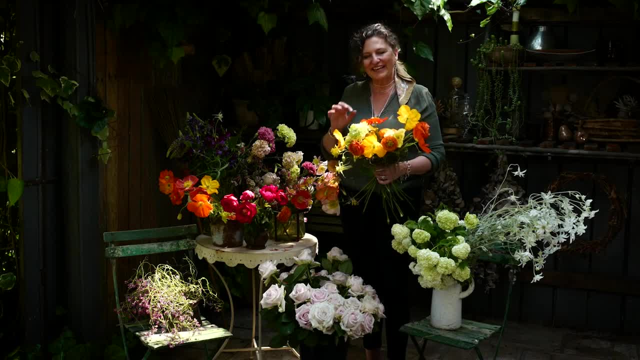 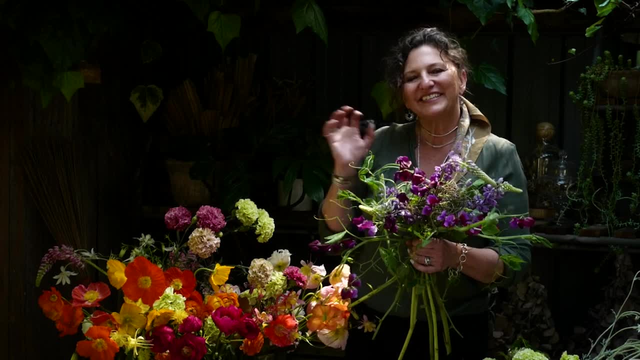 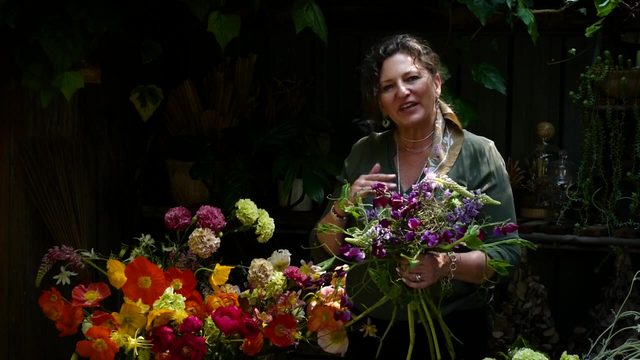 that bouquet I love. so, yeah, I hope you will consider an analogous color scheme, the three colors that are adjacent to each other on the wheel. with this color harmony, I wanted to share with you a complementary color harmony. so this is when we're looking at the color harmony and I'm going to show you how that. 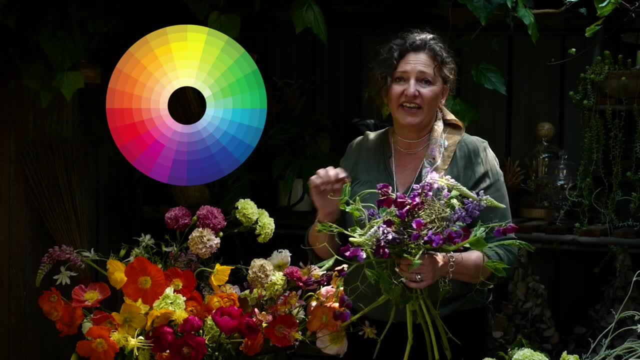 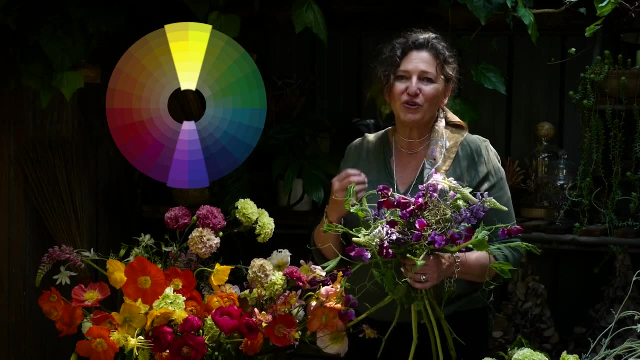 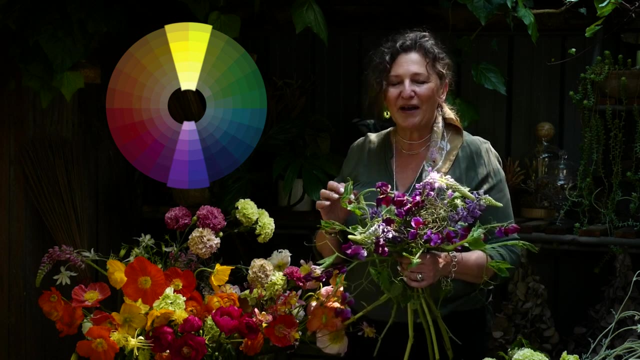 color wheel and we're looking at a color that's directly opposite each other. so for this instance, we're going to be using purple and yellow. now, nature does this beautifully. well, you might think that's a little bit scary. so we're really starting to delve into some interesting color schemes here. but but 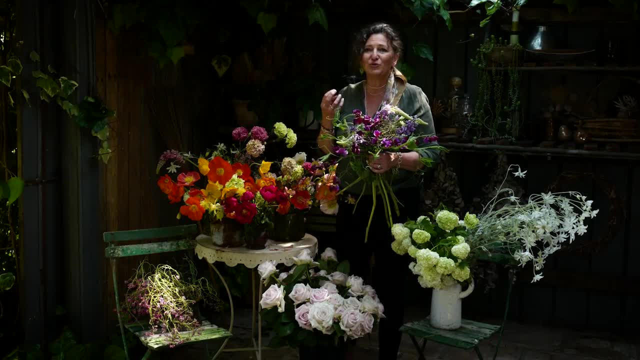 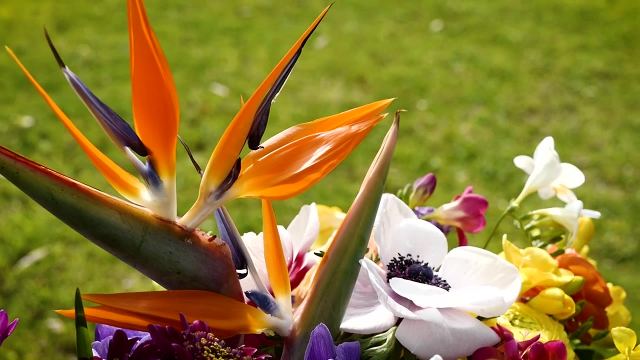 nature does this already. if you can think of a, a blue, purple Iris, you'll see there's a yellow stripe in the center. another flower that that's iconically complementary to the color wheel- and that's what we're going to be looking at- is a bird of paradise, and I mean, how amazing are they and so striking and so. 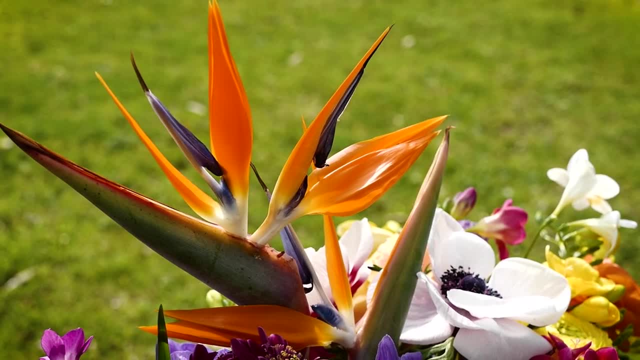 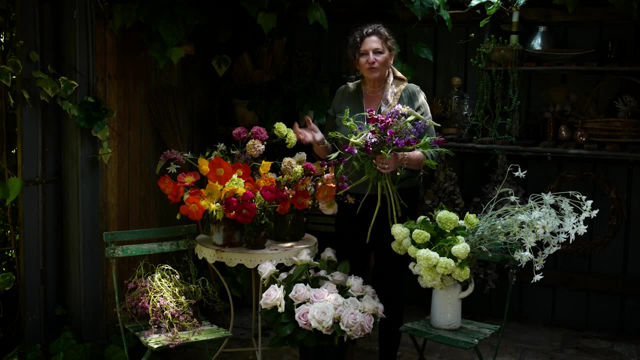 intense in their color and it works perfectly. so, really, I just want you to think of these color harmonies as a set of rules and guidelines to help you when you're designing, whether you're designing for a certain space and a certain aesthetic, or when you're, you know, putting together just your own. 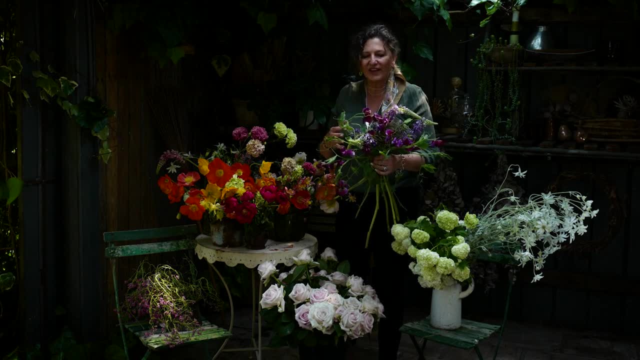 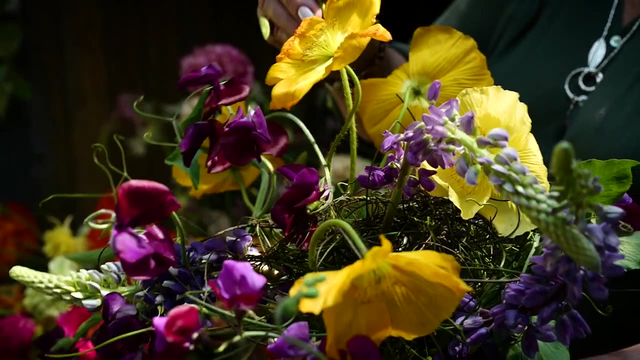 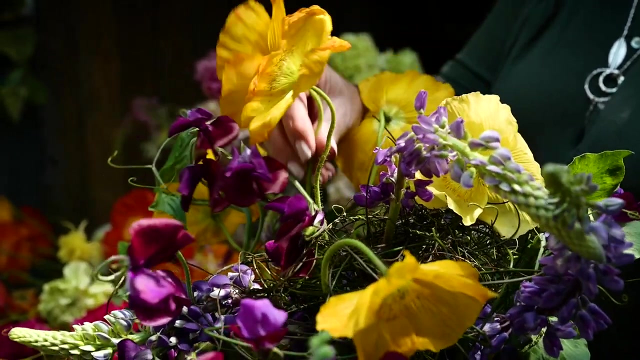 designs for your own home or for a client. it's important that you have a clear understanding of color. so with this one, you can see beautiful could be considered monochromatic right here, and we're going to bring in these pops of yellow and you'll see that it just 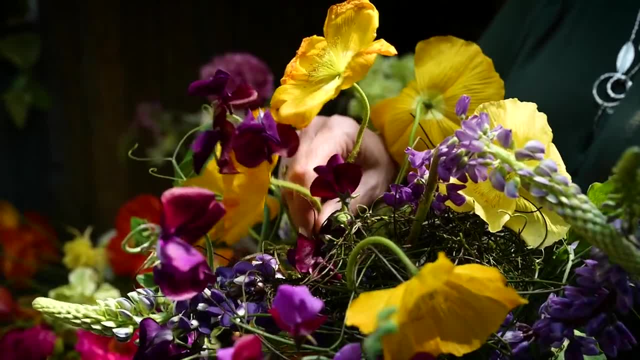 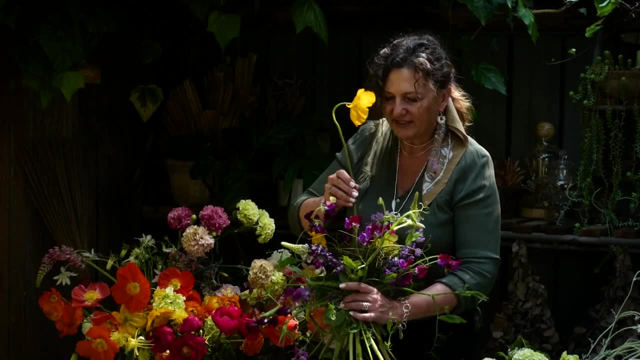 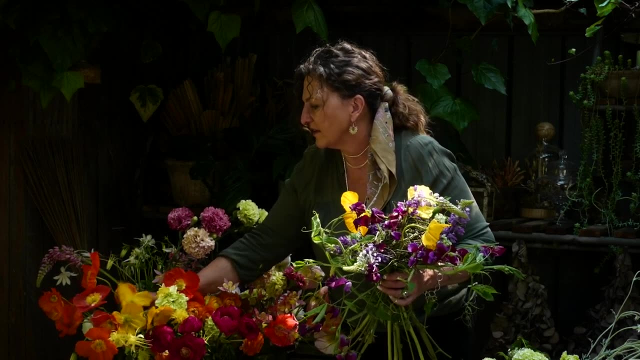 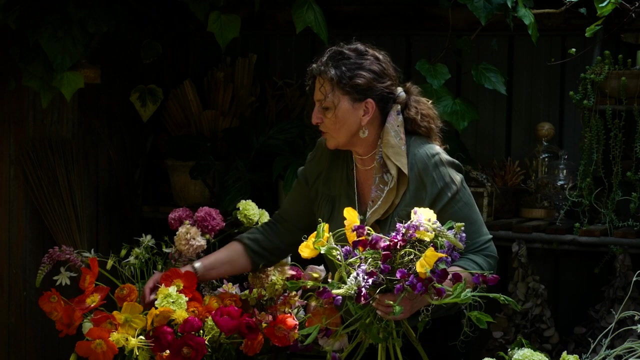 completely changes and morphs into something absolutely beautiful, I think, but a little bit surprising. and with having that set of those set of guidelines within understanding your color wheel and understanding of color harmonies, it opens up a whole new world of design for you, because you won't necessarily just get trapped into designing colors that. 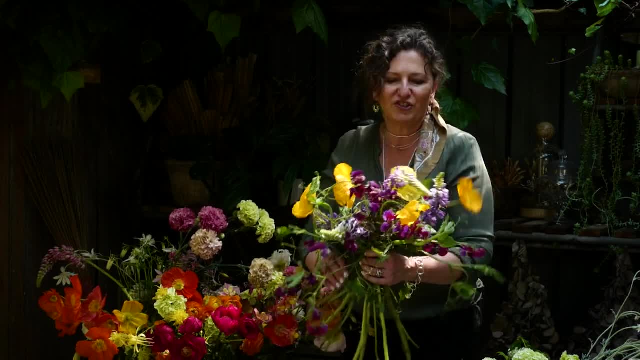 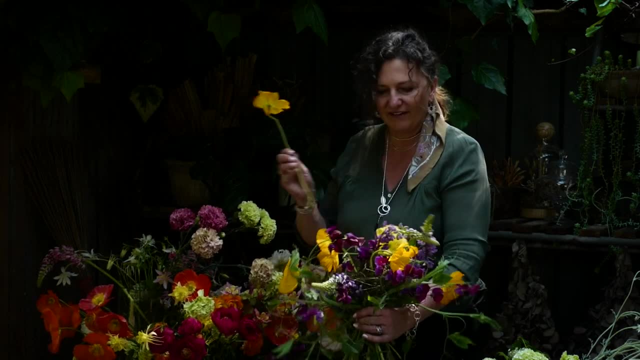 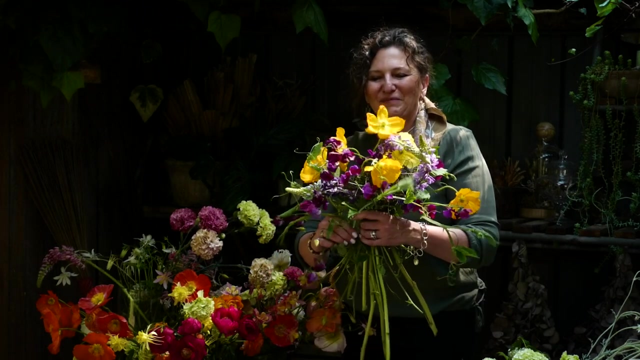 you'd like all the time. you know it's it's good to be able to stretch out and and do something completely different and you know I I love this together. I think that really you know they complement each other. that's why it's called a complementary color scheme. 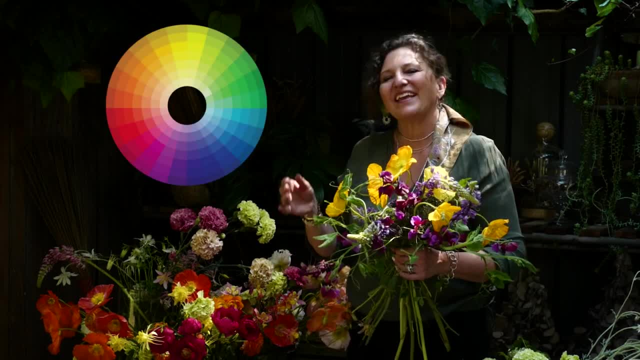 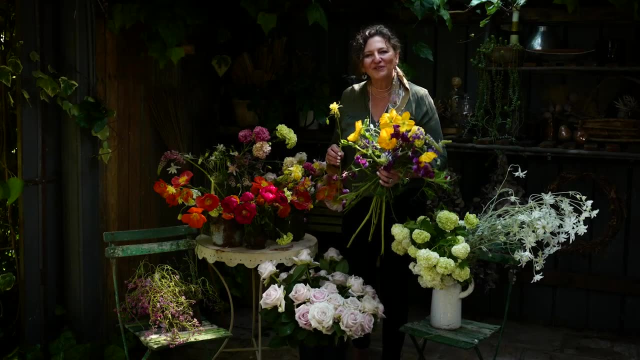 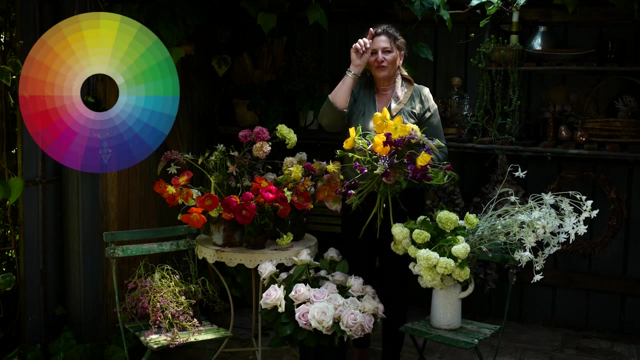 okay, so complementary color scheme, looking at the colors on the wheel that are directly opposite each other, and the final color, Harmony, that I wanted to talk to you about today is a split, complementary, and that's looking at three areas of the color wheel that are almost in a direct triangle and a great 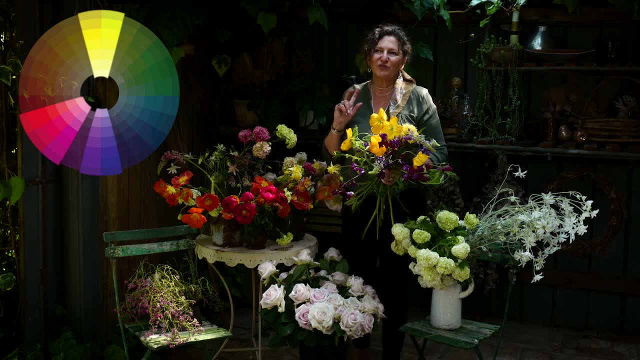 representation of how it's pressing, along with the color of the wheel. so this is like if you were to say, hey, do you know what those different colors look like? this school and the link bell and youtube working of that is my design, that you'll find much further up in the library and that 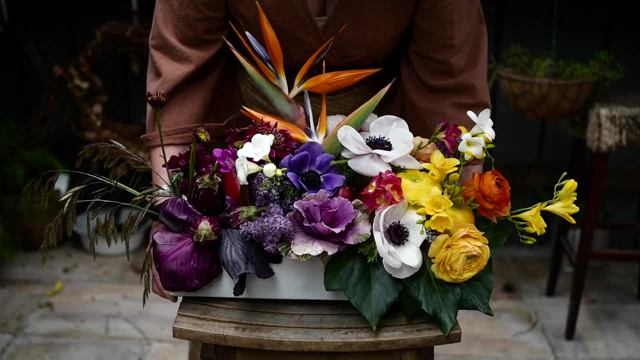 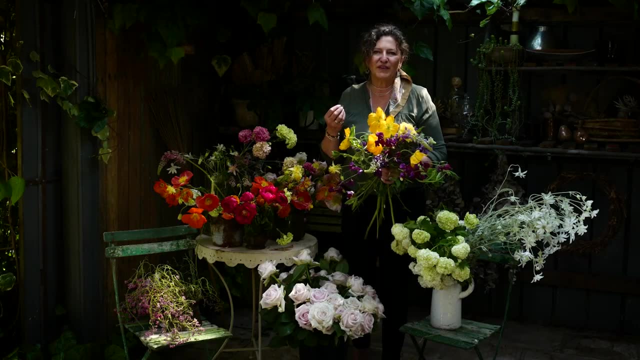 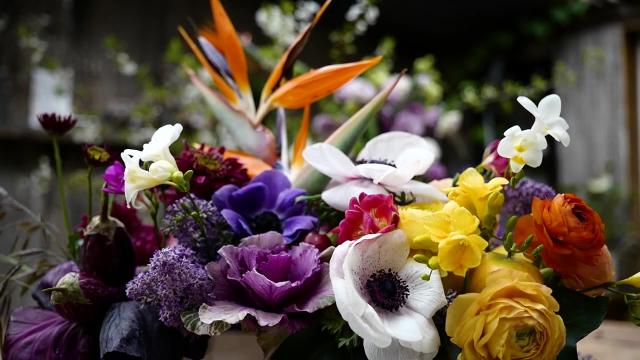 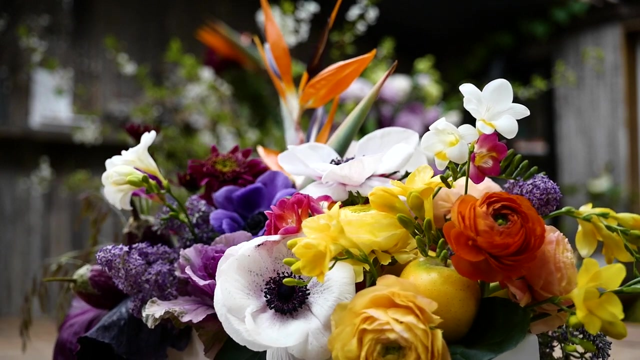 is my spring harvest centerpiece design. You'll see that we use a huge range of colors in that and basically a triadic or a split complementary color harmony is almost touching on every every color on the wheel. I guess it's the brightest combination that we can put together. So let's add just one more. 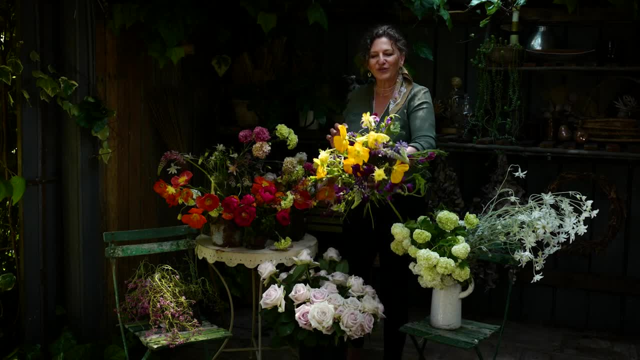 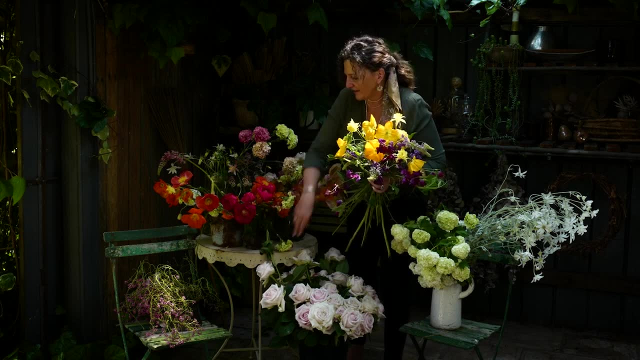 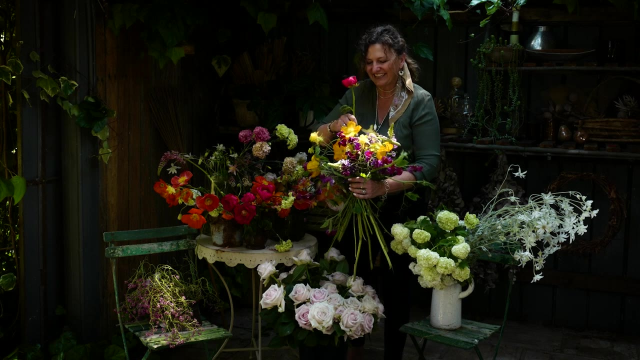 element that I, so I can show you how we can transform this complementary color harmony bouquet into a split complementary, and that's by bringing in these amazing peonies from Tasmania, the first, the first peonies of the season. It's always such a delight to have them and you can see now how that just 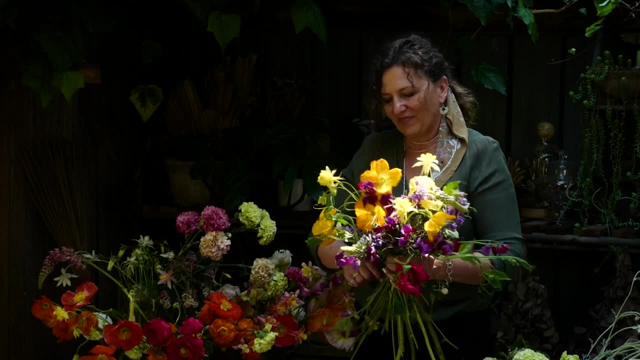 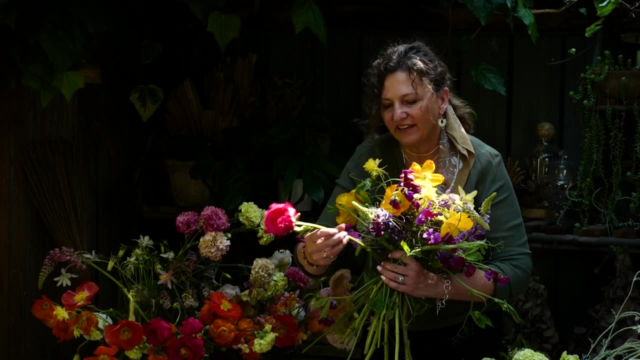 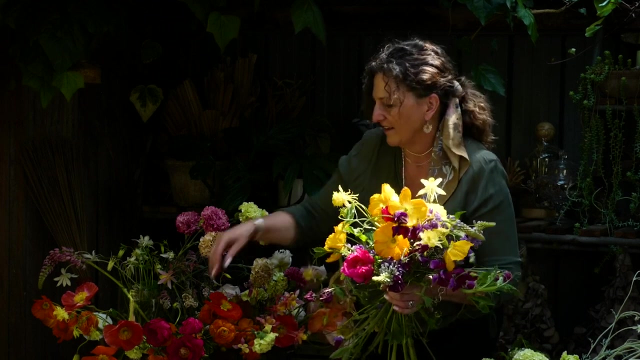 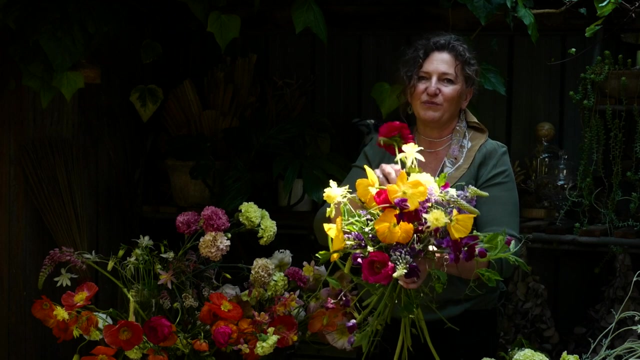 absolutely pops this bouquet. Also the fact that I don't know if you can see the center. the center is yellow. so by bringing in these, this gorgeous, you know, hot pink with yellow center peony, this transforms this bouquet now into a split complementary color: harmony. 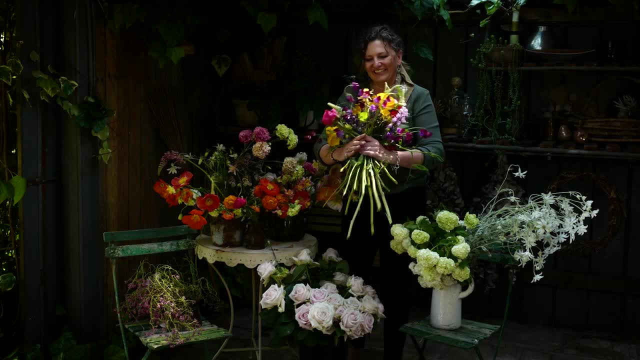 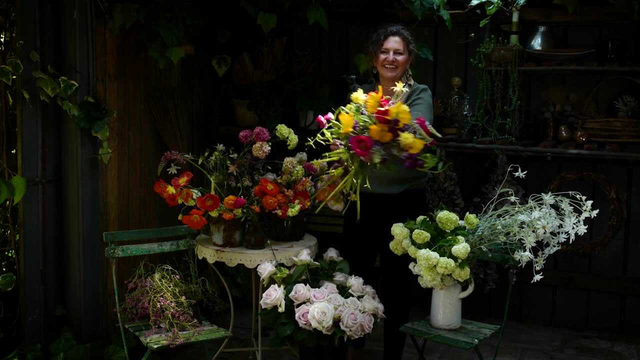 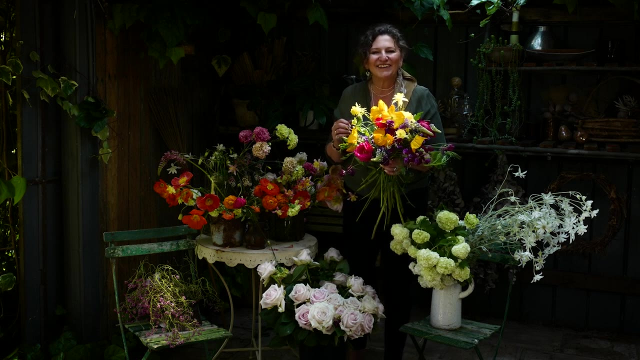 Okay, that's beautiful, don't those poppies, peonies, just pop in with all that other color around them, okay, so I hope this is allowed: you to feel brave by using color. it's important that you understand color as a designer and you're not just throwing things together.